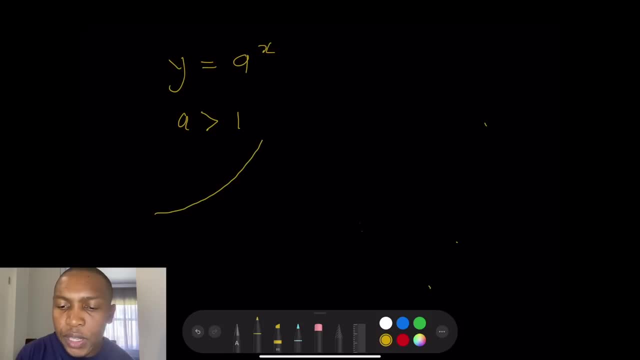 want you to note that increases obviously going that way. so this would determine the shape of the graph. but if the value of a um is less than one- okay, and of course it should be greater than zero in this case- then we know that the translation or, in this case, our graph, would actually be decreasing and this would be the shape. 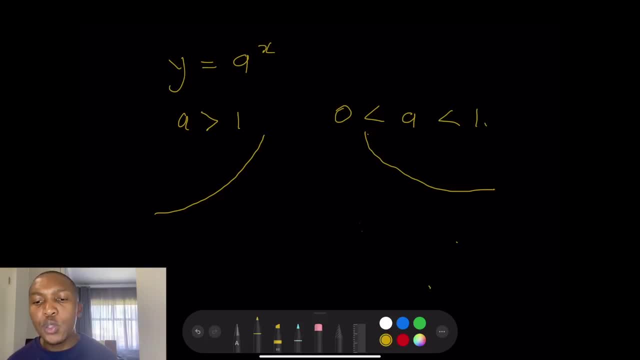 that goes along that direction. okay. so now a couple of things that you also need to know. um, remember for exponents any time that you've got anything to the power zero. okay, so if i've got a to the power zero, remember anything to the power zero. gives us one, and so that. 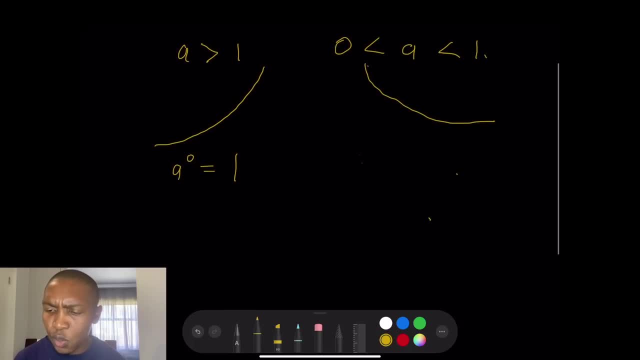 is why, for the basic graph: uh, i hope this color is not an issue, okay, so that's why, for the basic graph: uh, say, for argument's sake, we get y is equals to two to the power x. all right, what will that graph look like? okay, that graph will just simply be now remember. 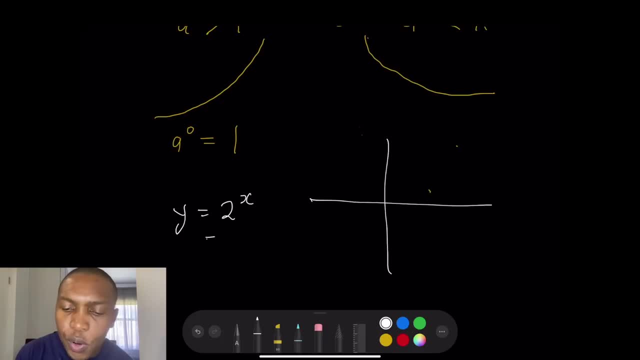 it should always cross whenever we've got two to the power zero. okay, that is equal to one. so meaning, uh, in our graph, anywhere where x is zero, that is in this case, where x is zero, we know that y will be equal to one. so our graph should cross there. you can see there that, um, you know, my, my, my. 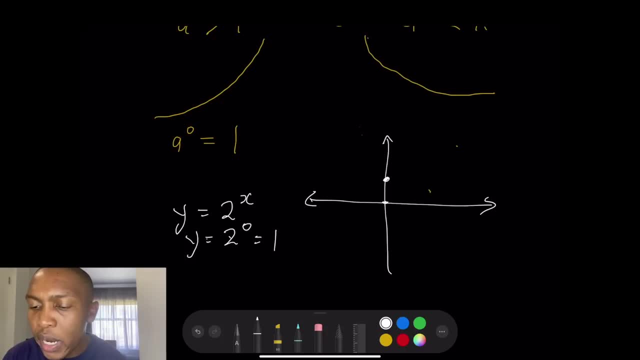 base is two, it's definitely greater than one, so the shape of our graph would look, uh, more or less uh, like that. okay, that's what our exponential graph would look like. now, just one other thing. so it means that for the exponential graph. now i'm not going to go into much of the pedantic details, i just want to get to the 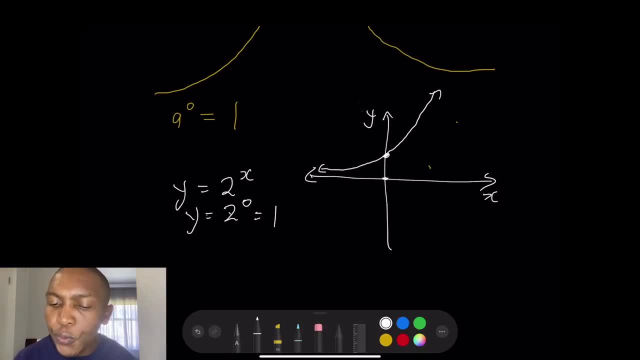 examples as quickly as we possibly can. so, for the exponential graph, what we want to do is i want you to please note that obviously now the y-axis- okay, rather the x-axis, rather the y-axis- will come and basically will now act as your asymptote, and you can obviously guess why. 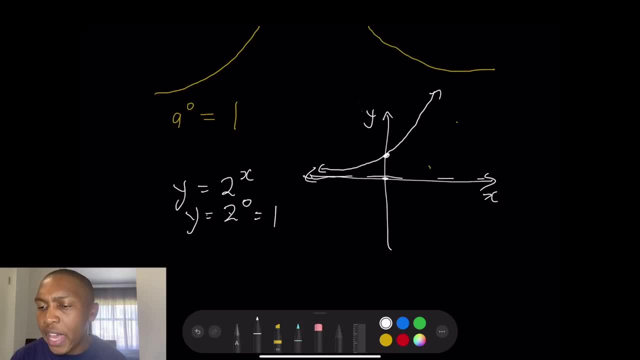 okay, because in this case that we, we cannot actually have the negative y, it doesn't matter what you do. so the, the, the horizontal asymptote in this case, would become uh. y is equal to um, or rather i said horizontal as into it, but i'm writing why. 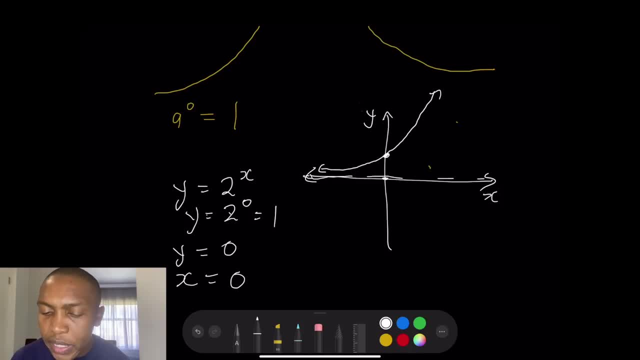 equal to zero. okay, so in this case it means that for our horizontal asymptote we've got: x is equal to zero, so it means that the graph will never cross that line. okay, right now just a couple of things to note there. if we were to have a translation, maybe before i get even to. 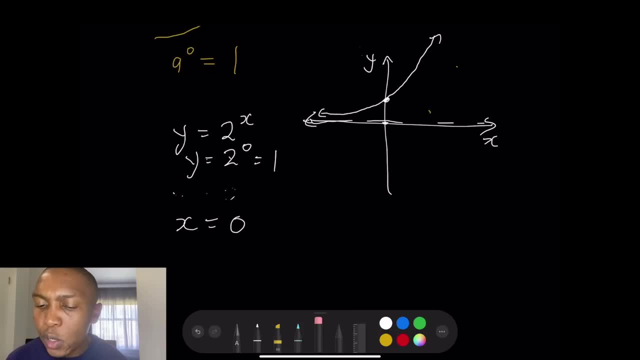 that okay. i want us to look at what the graph looks like when it's shifted, and i'm just going to make some comments about that. so in this case, the equation can change as follows: we can have: y is equals to a into x minus p plus q, and please i want you to note what that simply means. 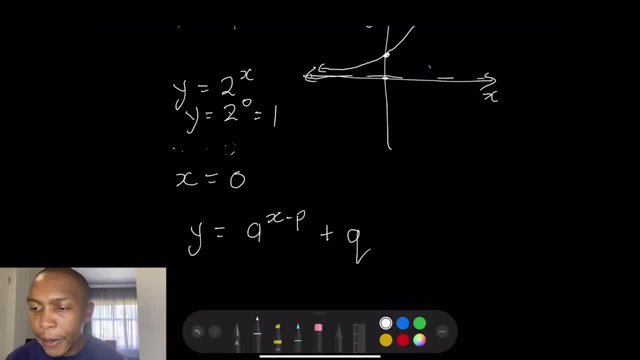 it would be the same graph that we had, okay, the one that we drew there, but what is the difference? it means that we are shifting. now, please, i want you to note this. when p, the value of p, is greater than zero, okay, so in this case, when p is greater than zero, it means that we are shifting. now, please, i want you to note, it's x minus. 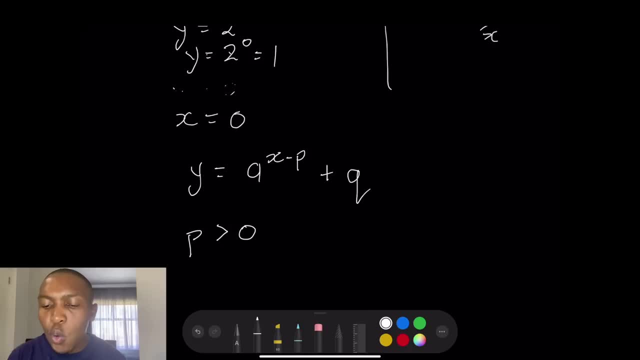 p. right, so it's x minus p. when p is greater than zero, it means that we are shifting our graph to the right. okay, and of course, when p is less than zero, it means that we are shifting our graph to the left. okay, so that means, if we've got in our previous example, suppose we have y. 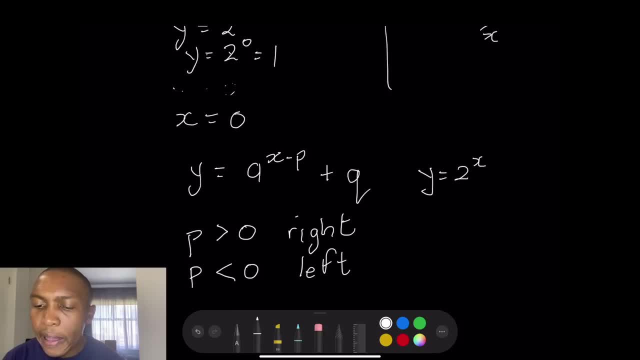 is equal to 2 x minus 1. note that we already had a negative sign for p in the place of p there, so it's x minus 1. so what would this translate to? it means that we are taking the very same graph and we are now shifting it to the right, in this case by one unit. okay, so whatever happened at zero. 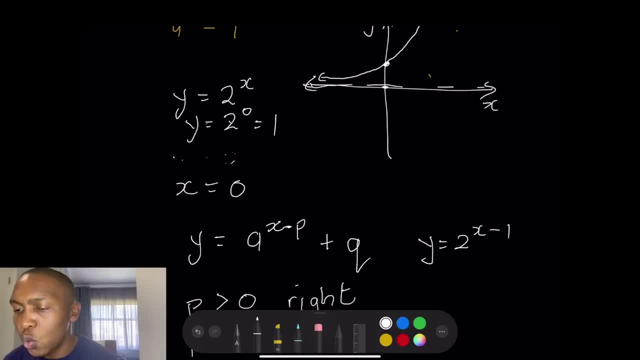 would now happen at? x is equals to 1, okay, right now. for q, on the other hand, okay. so this, this is what we would call sorry for p. let's, let's go for p first when we're talking about shifting to the right and to the. 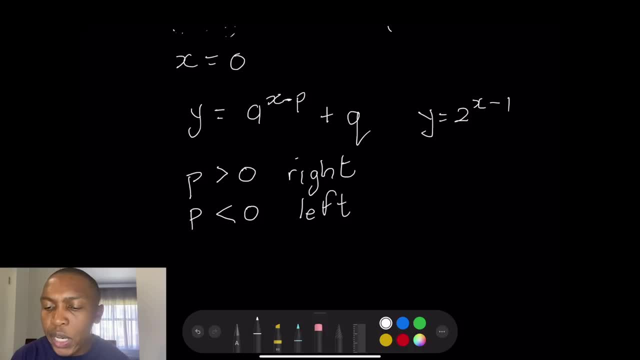 left when p is greater than zero. we said: we are shifting to the right, okay, and so that means that this is what we call a horizontal shift, and obviously we are shifting to the right, and so that means that this is what we call a horizontal shift, and obviously. 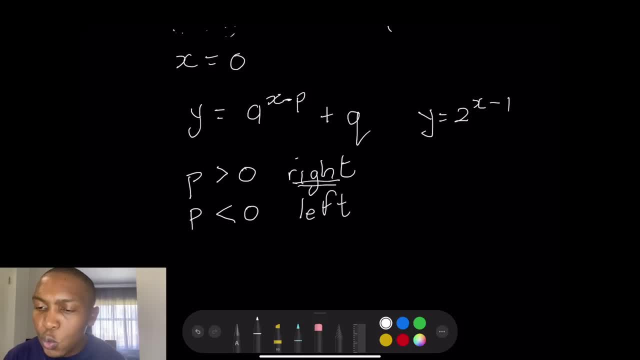 shifting to the left or to the right. now, when q, this value over here. all right, i'm just going to circle it with a green. so when q is greater than zero, in this case, then what are we doing? we are taking the same graph and we are shifting upwards or downwards, right, but in this case, when q is, 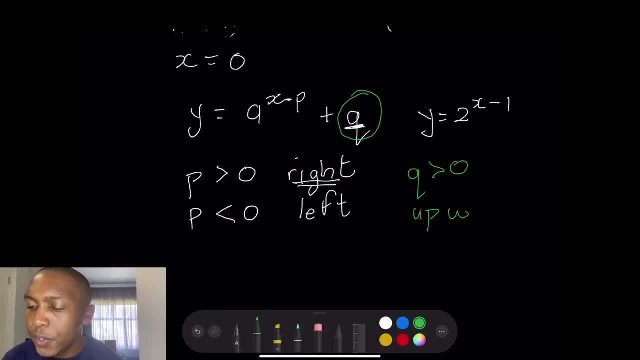 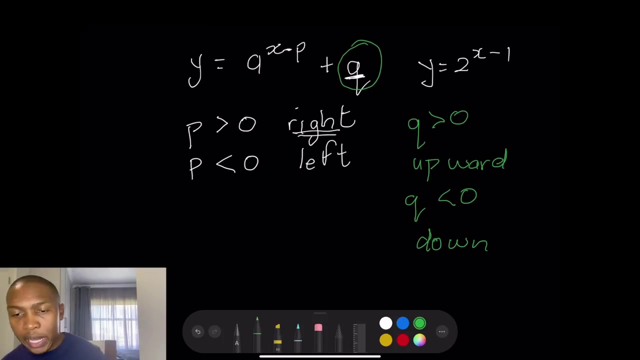 greater than zero, it's an upward shift, okay. and again, when q is less than zero, okay, so it's a downward shift, all right. so what i would like to get to, ultimately, is that we should get to a point where we can do some examples on this. 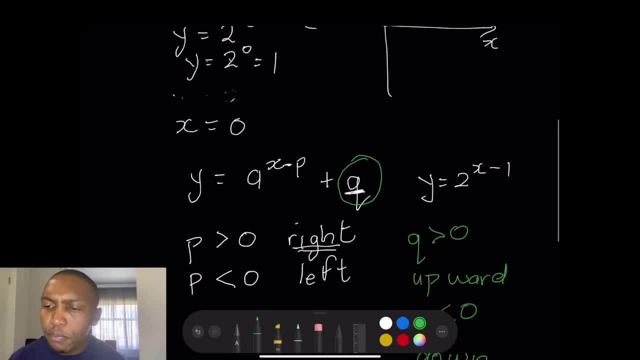 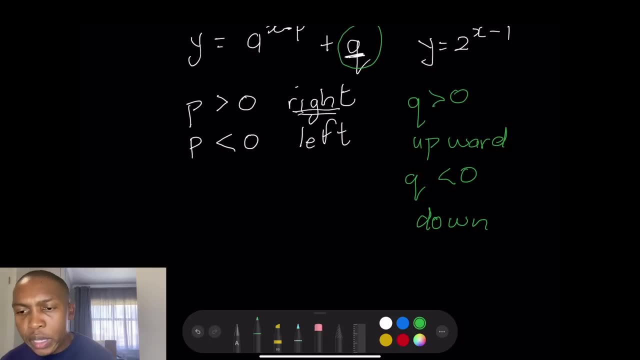 okay, um, just um, what else do i need to mention, uh, in terms of this graph? okay, uh, so we can find x intercepts and y intercepts. we'll get into that. i think i want to mention that once i've got my examples. um, yeah, i think let's just dive right into an example and see. 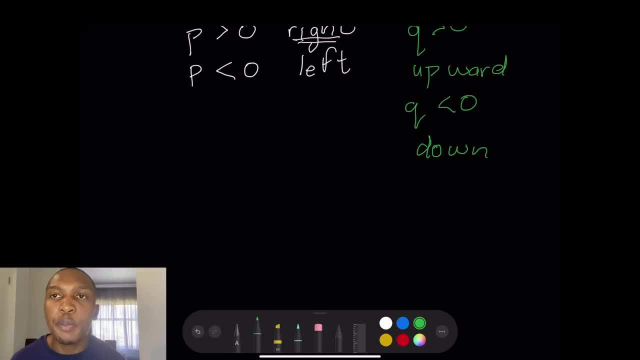 how to apply when it comes to the exponential graph. all right, so now we are going to look at, um, just how to draw the graph, and i don't want this video to be too long. let's just get straight to the point. okay, um, of course, you know we could have had, uh, just a. 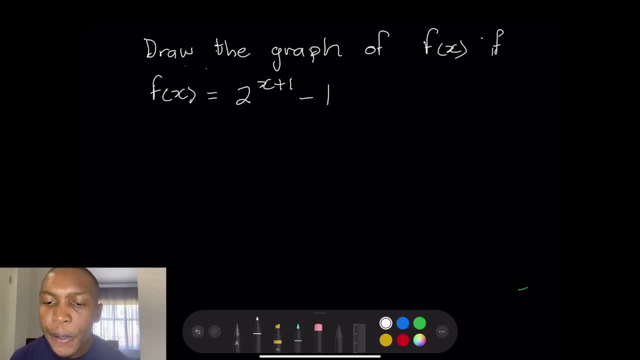 situation where we don't have shifts. but i want to include them now because you know the other graphs can be quite straightforward and simple, right? so now they say: draw the graph of f of x. if f of x is 2x, 2 to the power, x plus 1 minus. 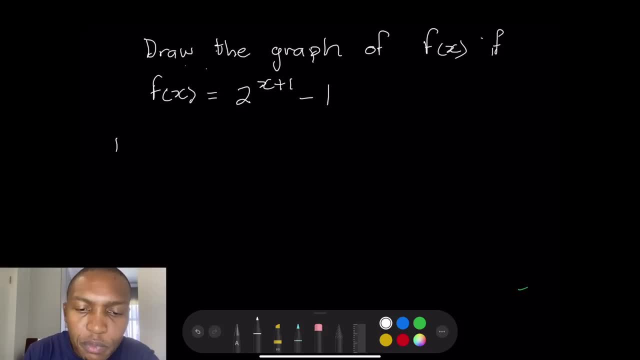 1. so the first thing that we're going to do is let's note what they've done. they've taken a graph. our base is 2, okay. so meaning that when we know that our base is 2 in this particular case, then we know that we are going to have a graph that increases as you move towards the right. 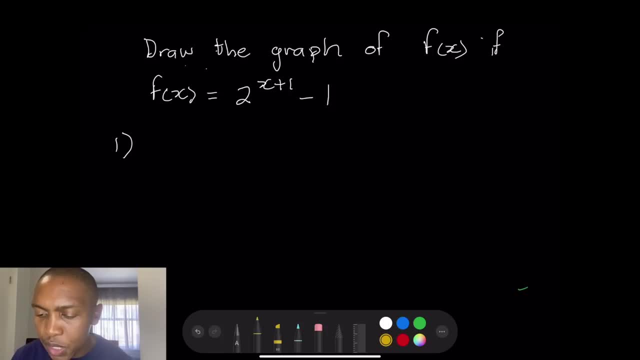 but what have they done? they have shifted. now let me just use another color. all right, they have shifted it. okay, so we're going to have a graph that increases as you move towards the right- okay, in this case we've shifted the graph- and to the left. so when we see a positive there, 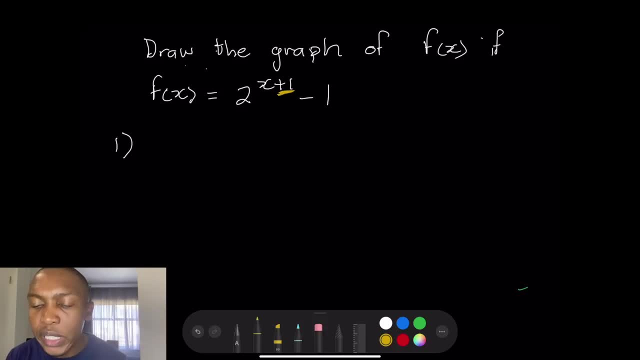 it means we have shifted it to the left by one unit. okay, so if you had a graph of 2 to the power x, we've taken the graph of 2 to the power x and we've shifted it to the left by one unit. but we've also taken that graph and we've shifted it. now note this: minus 1, it means we have shifted. 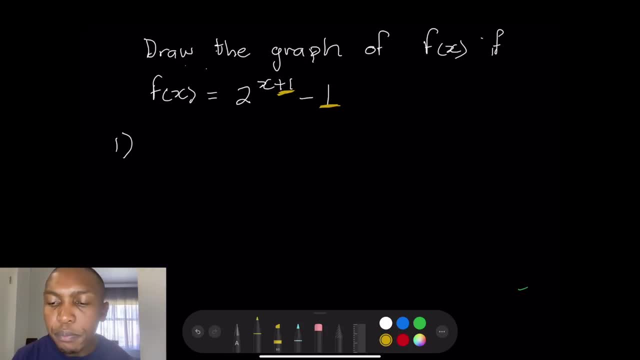 it down by also one unit. okay, so now remember, as opposed to having the graph being okay. so if it was a just a normal graph, it would look: uh, something like that. we know that, uh, y, i mean x, is equals to 0 would be our horizontal asymptote. okay, that line over there. okay, let me make it red. so that line would be. 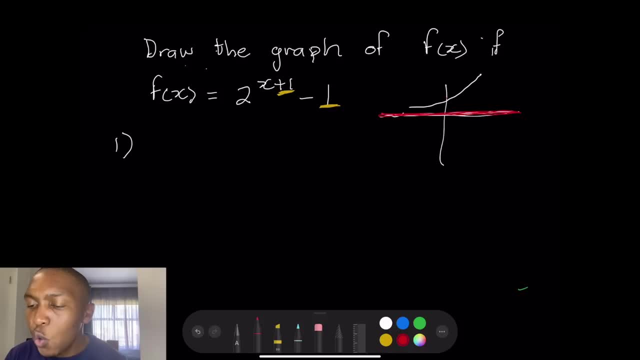 a horizontal asymptote. now it's no longer going to be a horizontal asymptote, but instead- uh, let me just choose the yellow color, right instead? minus 1 is going to be our asymptote because of that- um you know- vertical shift. it's been shifted vertically. 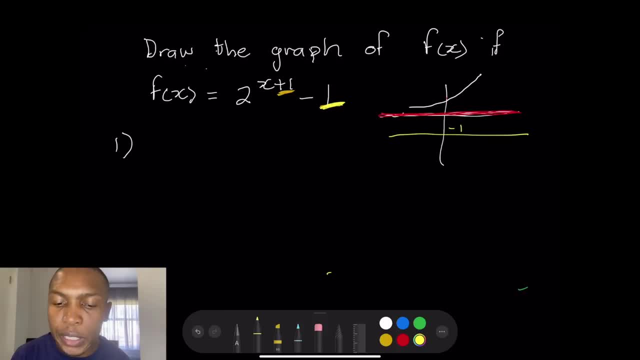 by one unit, so we've shifted it down by one unit. so what is going to be our asymptote in this case? we start with our asymptote, so our asymptote is going to be at x, uh, actually, y, um. yeah, this thing can show you proper flames, eh, uh. so that's going to be at y. 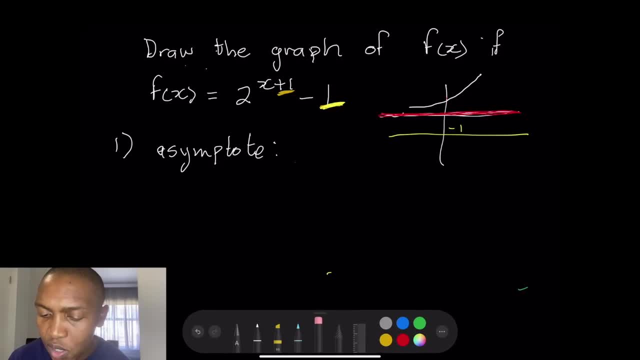 is equal to all. right, our pen is not behaving again, so this is going to be: y is equal to minus one. okay, so this is where our horizontal asymptote lies now. secondly, let's do this, let's find the x intercept and the y intercept now, please. 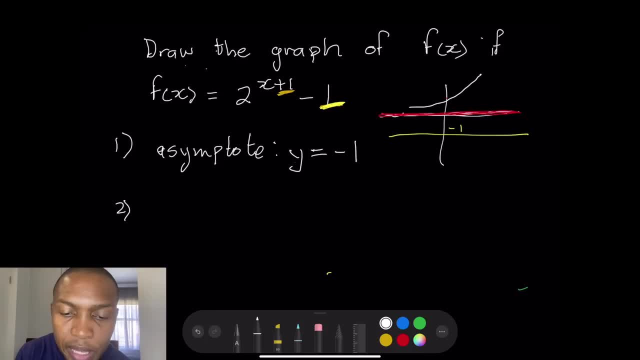 remember, i haven't drawn the graph as yet, i was just illustrating something there, so let's find the x intercept first. okay, now remember what happens at the s x intercept. we know that y is equal to 0, so it means that i'm going to take that graph, okay, and say 2 to the 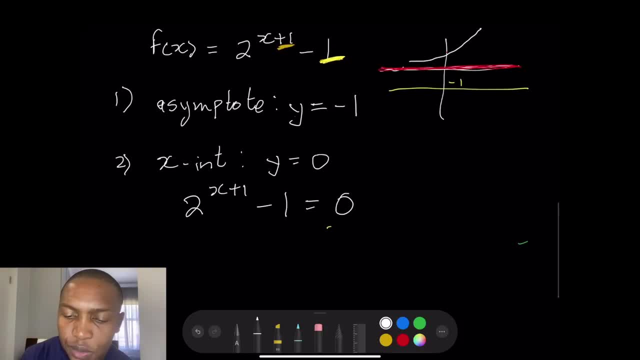 y is equal to 0, okay, so let's try and solve for that. so this is going to be 2x, sorry, 2x plus 1 minus uh, or rather is equal to 1.. so what we do when we are dealing with exponents- and of course, we're going to get to a time when we just deal with exponents- 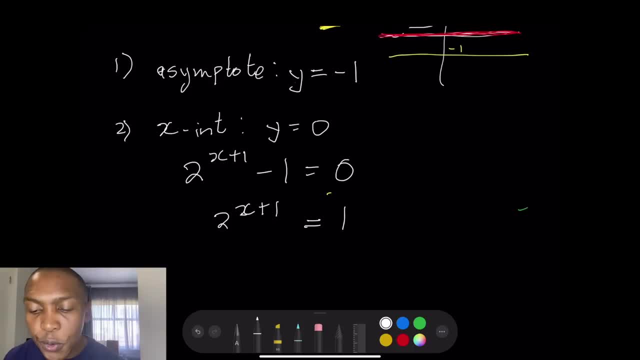 i know, because you know we're trying to uh cater- for you know metrics at the moment, but we'll get to that time where we deal with exponents. so what we do, we try to get the basis to be the same. so in this case i've got 2x plus 1.. um, in this case i can say 2 to the power. 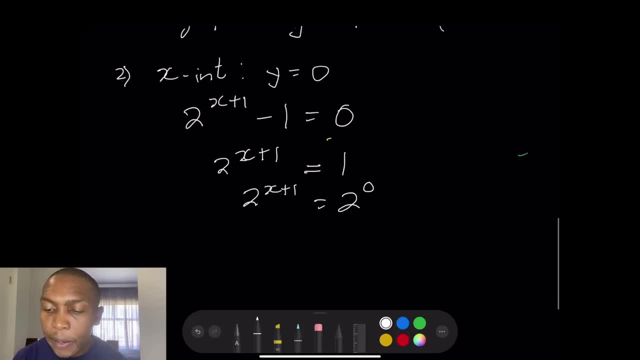 0. remember anything to the power? 0 is equal to 1.. so, as a result, if my bases are the same, i can drop down the exponents. so in this case it's x plus 1 is equal to 0 and therefore it means that x is. 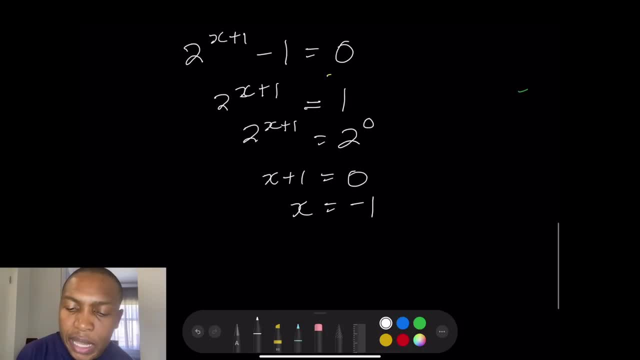 minus 1.. so remember what this simply means is that our graph is going to cut through the point minus 1 and 0. okay. and then we find the y intercept. okay, so we find the y intercept. okay. remember what happens at the y intercept. we know that x is equal to 0.. 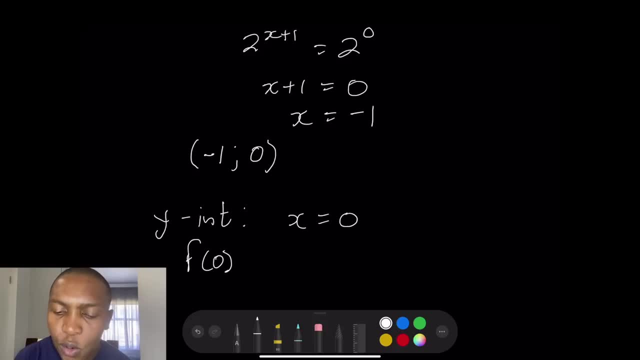 so it means that we're going to take our f of 0. everywhere we see x, we are going to do it with 0.. so remember, so this is going to be 2 to the 0 plus 1. okay, minus 1. so what do we? 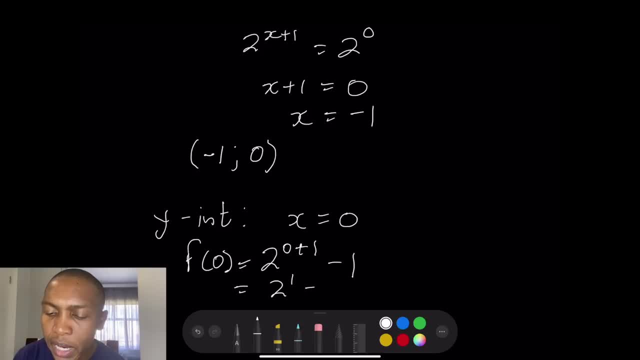 actually have. we have 2 to the power 1 minus 1, and remember, 2 to the power 1 is 2 and, as a result, that remains two. uh, sorry, that remains one. what happens to my maths? okay, so that becomes one. okay, so our gets. 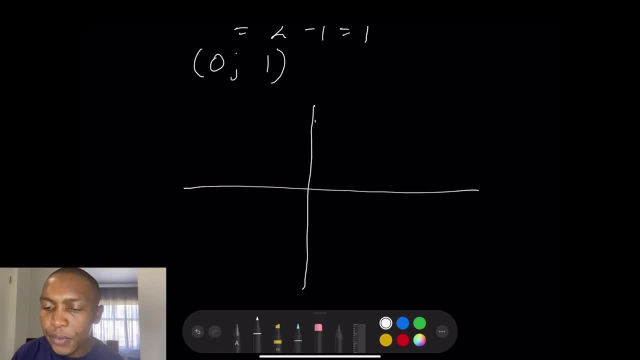 equal to 0. okay, so it means that our graph is also going to cut through the points where x is 0 and y is 1, right? so what does this translate to? let's try and draw a graph, okay. so there's our graph there. okay, these are my axes. 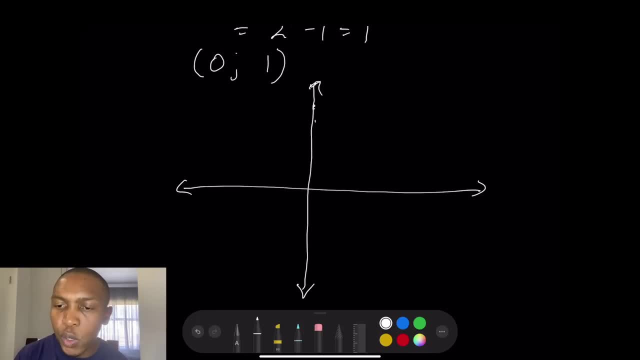 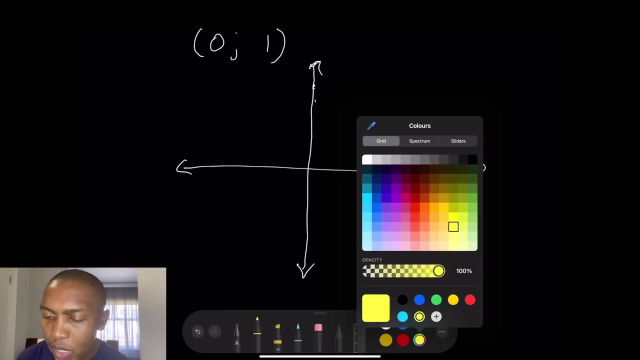 okay. so in this case, what we are going to draw is we just need to put our x up and down to do is we know that our graph is going to cut through, or first of all, let me draw the asymptote. okay, we said we're going to have an asymptote. let me make it nice and bright. okay, we said we're. 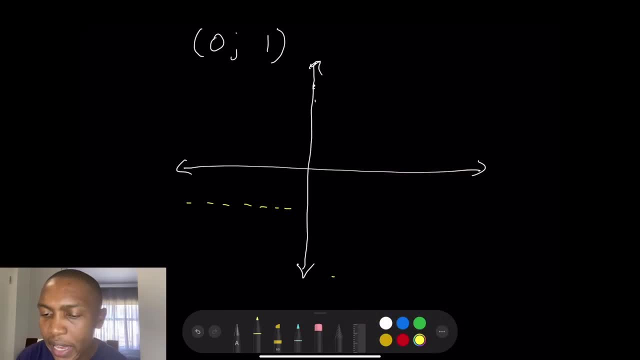 going to have an asymptote at y is minus one, so our graph will not cross this line. and then, secondly, our points. in this case, we are going to have a graph that cuts through minus one and zero, okay, so where x is minus one and y is zero, okay, so let me make that nice. and 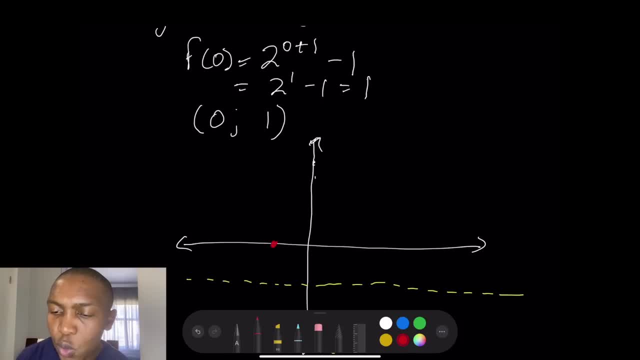 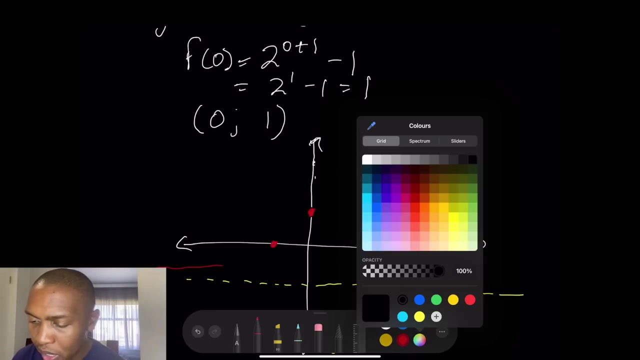 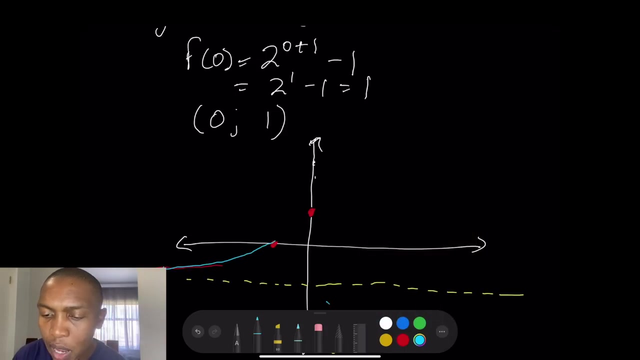 red, okay, and then we are also going to cut through the point where x is zero and y is one, okay, okay, um, instead of making that red, i actually took off there, all right, so there's our graph. in fact, let me just choose another color. okay, i want something which is a little bit brighter. okay, so our graph would look something. 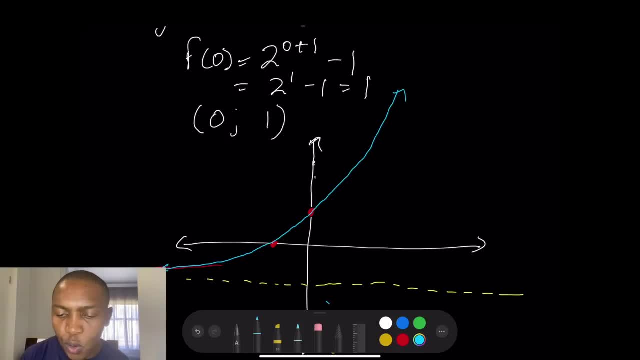 like this. okay, so we know it would never cut through, uh, in this case. so that's our x and that's our y, and in this case, that would be our graph. okay, right, so i hope that makes it quite simple in terms of the exponential graph. now just a couple of things. um, i know i 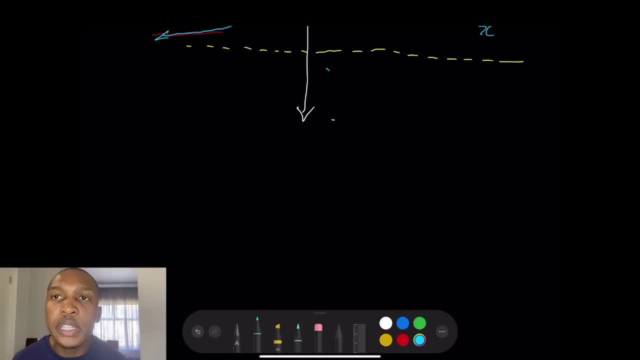 haven't spoken much about this because i wanted to treat it more or less, you know, separately, but i am going to actually treat it at a point because i want us to talk about reflections and you know, um, you know symmetry, but we will actually treat that separately. however, for the exponential graph, let 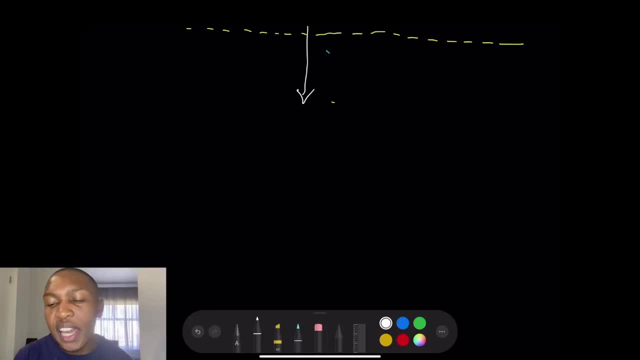 me just, you know, get ahead of myself a little bit and then, um, i'll just come back and obviously add more detail. so if, in this case, suppose, i had a graph, uh, let's say, y is equals to 2x. okay, remember, in this case where i 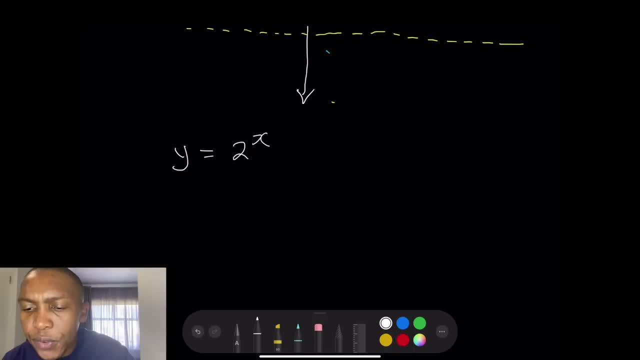 now want to, to have a translation. now, what would this graph looks? look like it would be a graph. remember? we said it would be a graph that looks like that and i know it would cut through zero and one. okay, where x is zero and y is one. now what would happen if i wanted to draw a graph? okay, y is equal to two. 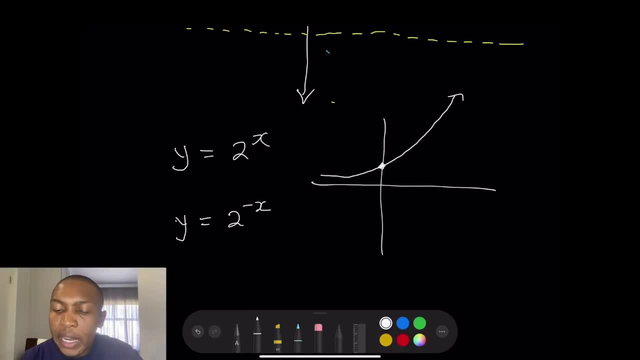 to the minus x. do you see what i've done? i've actually made now- uh, you know, translated this graph. so instead of having positive x, i have now a negative x. now, please, i want you to note once i do that, okay, what happens is that it becomes a graph. that is now. 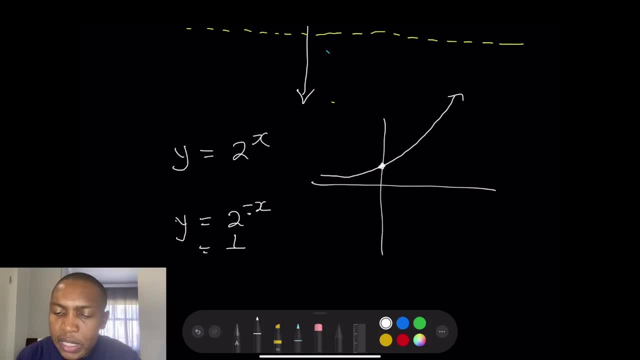 um, so two to the minus x is the same as saying two, okay, two to the minus, one to the power x, and which is the same as one over two to the power x. so what we've in fact done, you see, now i've actually taken away space for myself. 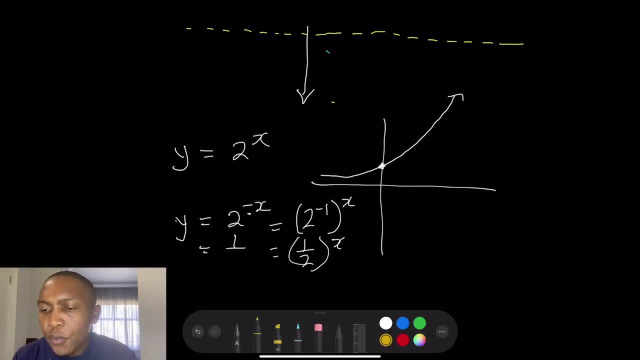 okay. so what we've actually done is that, if you remember what we said earlier on that, when the base is actually between zero and one, what simply happened? it means that the graph is actually going to be decreasing as you go that that direction. so once i make x, once i change the sign of the x, in this case, it becomes a graph that is mirrored.